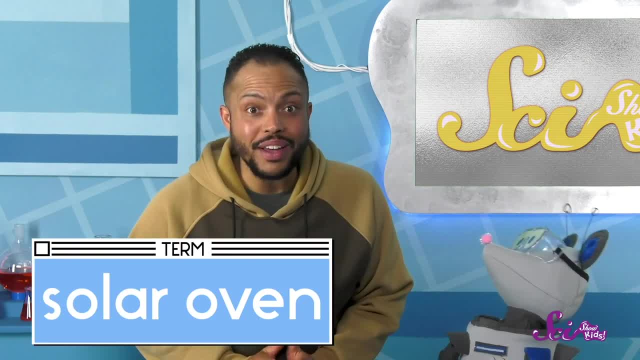 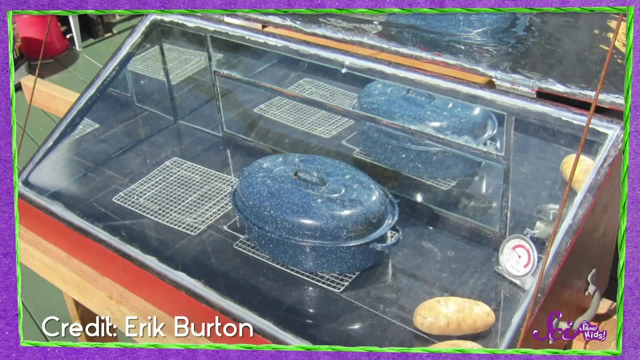 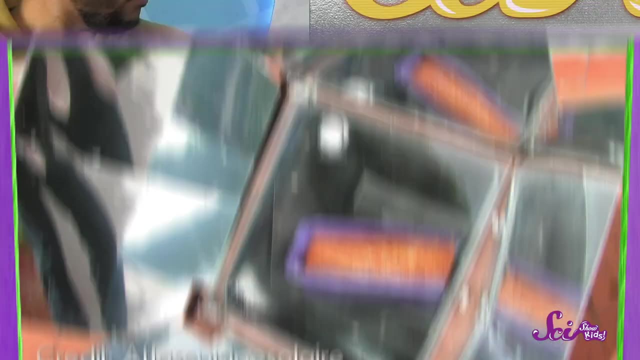 I know We can build a solar oven. Solar ovens are a lot like kitchen ovens. They're basically boxes that heat up inside and that are great at keeping the heat trapped inside of the box. If you put food inside of the oven, the heat cooks the food. 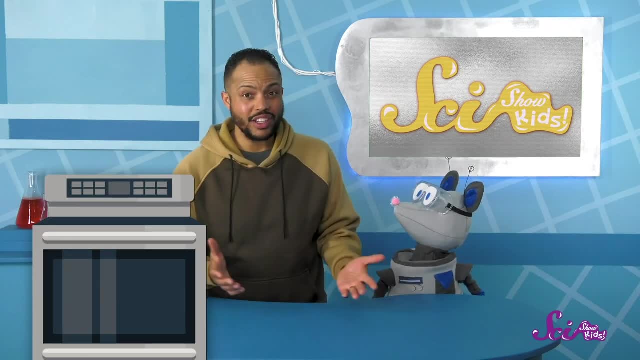 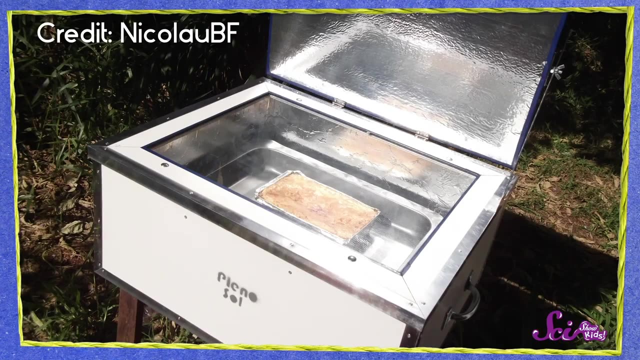 What makes it a solar oven? Well, kitchen ovens use electricity or burn gas to make themselves hot. A solar oven uses solar energy or energy from the sun. When light from the sun shines into a solar oven, it heats up the inside of the box. 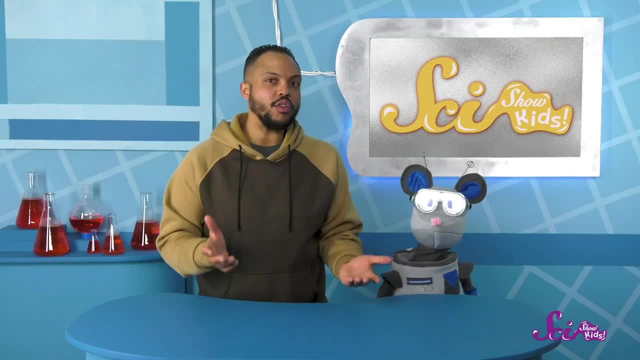 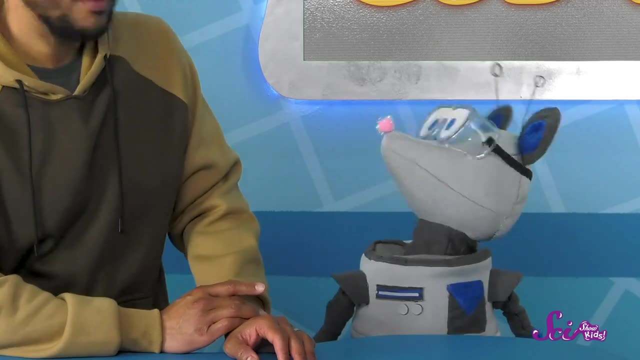 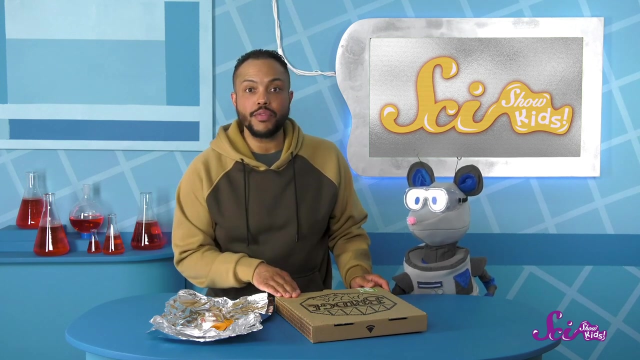 This means they're perfect for cooking outside. You can make a solar oven using materials you might already have. Hey Squeaks, will you help me design our oven? Awesome, I've brought some materials for us. First, we have a pizza box to use as the main box of the oven. 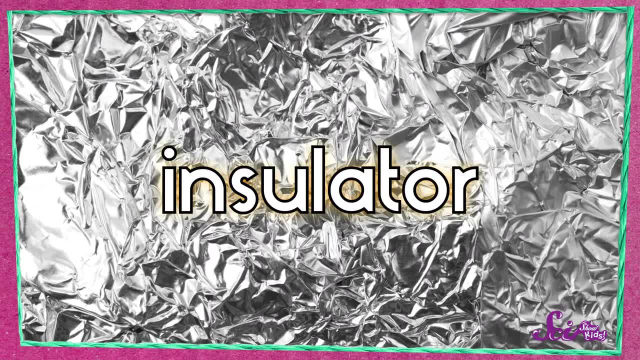 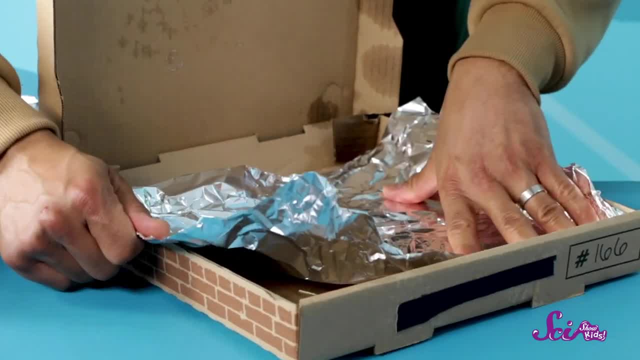 And I have some tinfoil too. Tinfoil is a great insulator or something that's great at trapping heat, So it can help us to keep the heat inside the box. I'll cover the inside of the box with tinfoil. 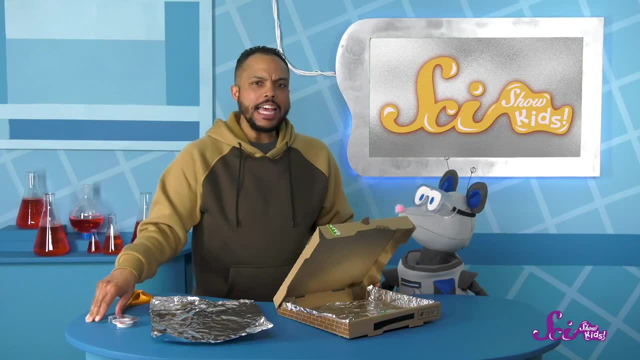 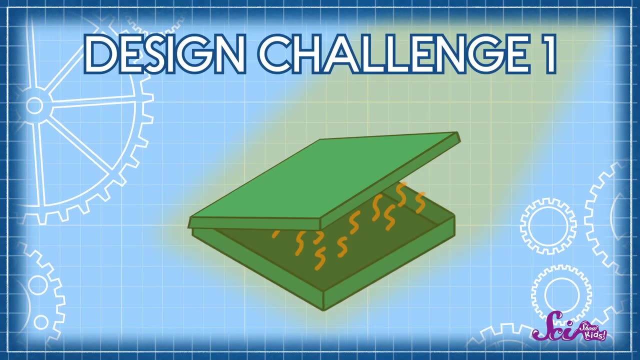 And tape it down. Hmm, Now we have our first design challenge. We need sunlight to get into our box, But if we open the box, all the heat will get out. Is there something that we could change about our box to get sunlight in while still keeping? 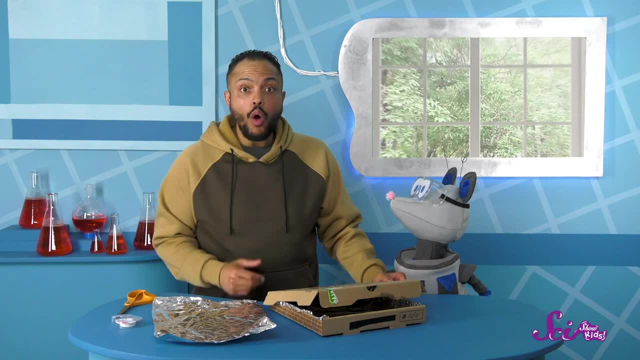 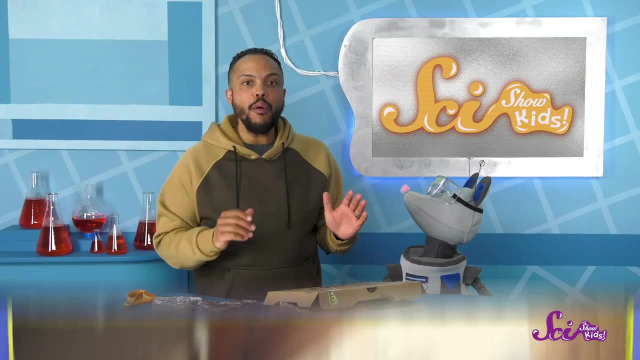 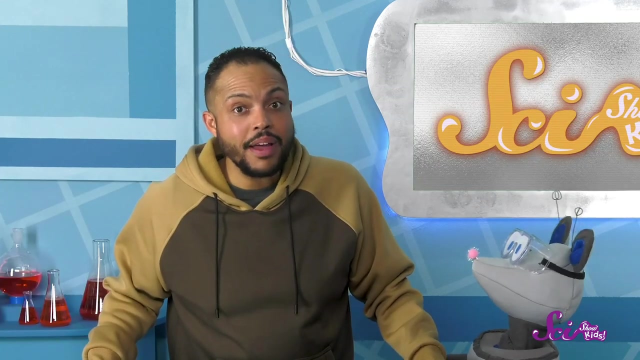 the box closed A window, That could work. It will be like how windows can let sunlight into a building even if they're closed. I'll make a flap so we can open and close it, And kids make sure that when you're cutting your flap, that an adult is around to help. 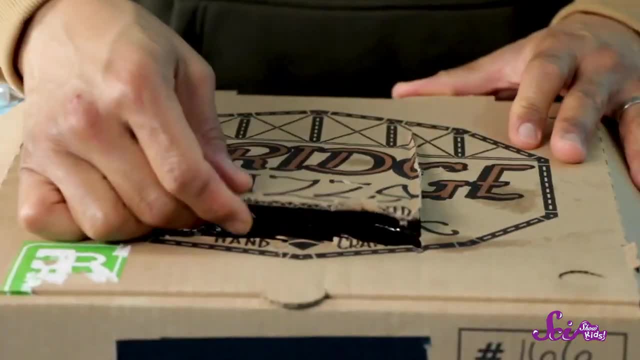 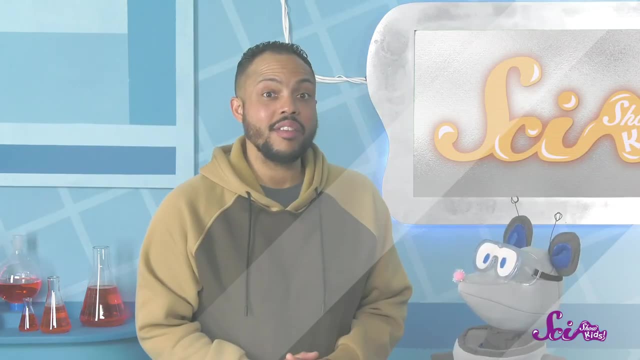 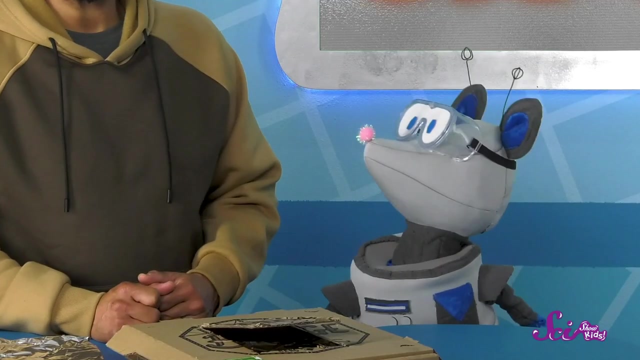 you. Normally, windows use glass to separate the inside and outside. We want something clear, like glass that will let sunlight in but that doesn't break as easily. What do you think we should use? Plastic wrap is a great idea. We can cover the window in plastic wrap and tape it around the window. 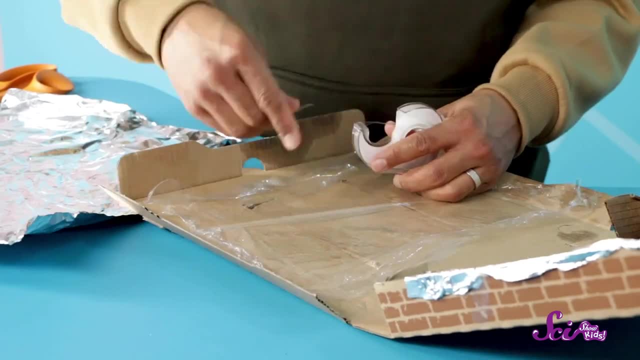 We can cover the window in plastic wrap and tape it around the window. We can cover the window in plastic wrap and tape it around the window. We can cover the window in plastic wrap and tape it around the edges to keep the heat inside the oven. 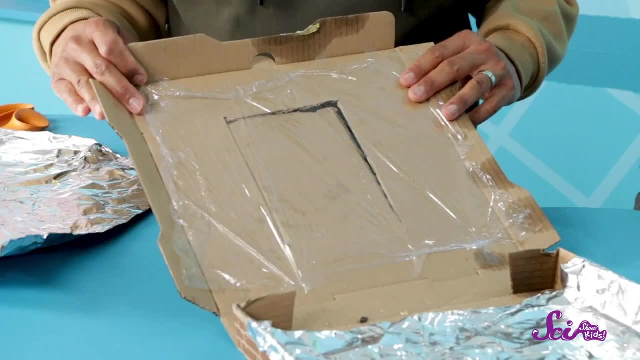 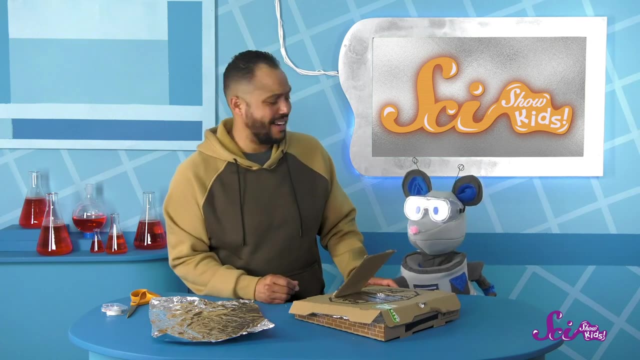 We can cover the window in plastic wrap and tape it around the edges to keep the heat inside the oven. Now sunlight can get into the oven and heat up our food. Uh-oh, I think there's another problem with our design. The only sunlight that can get into our box is the light that shines straight into our 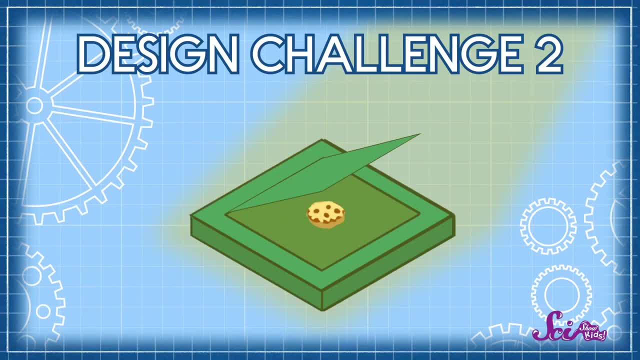 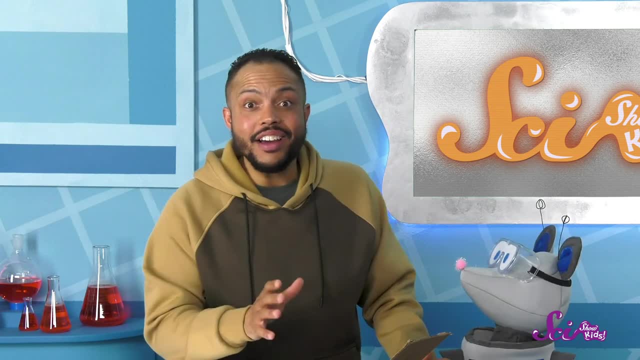 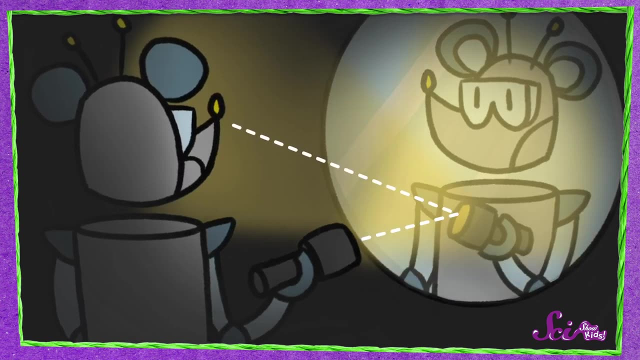 window. And that's not enough. So here's our second design challenge: How can we get more light into our solar oven? I've got an idea. Did you know light can bounce? I've got an idea. If you shine a flashlight in a mirror, the light will bounce off it and back at you. 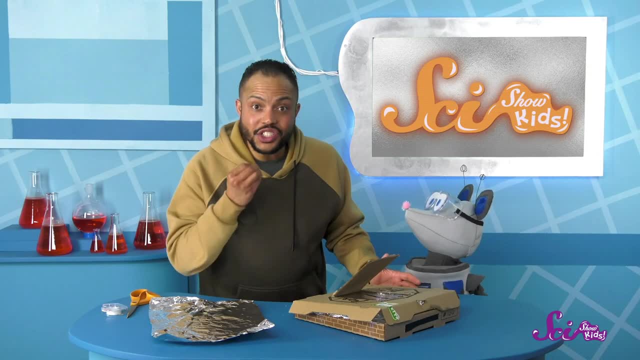 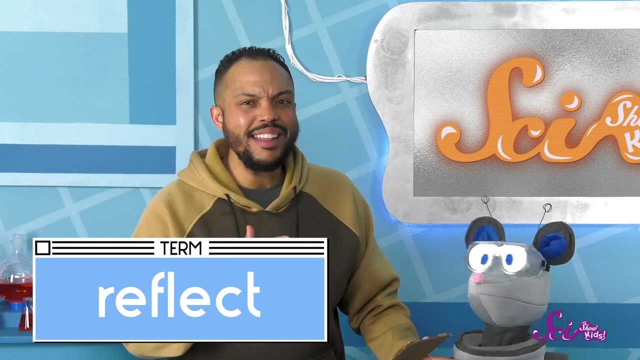 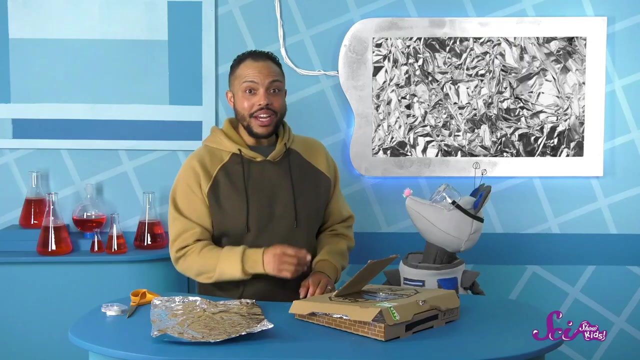 And it does this on more than just mirrors. Anything with a shiny surface can make light bounce or reflect, So if we want to reflect some sunlight into our solar oven, we need something shiny- The tin foil. The tin foil is very shiny. 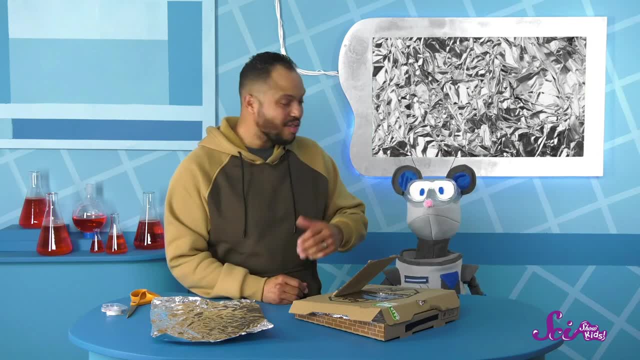 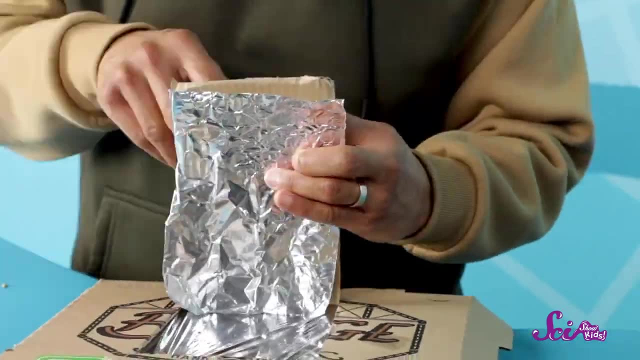 We can try using that to reflect the sunlight into the box. Thanks, Squeaks, I'll tape some tin foil to the box. We can also tape some tin foil to the section of the lid we cut out to make our window. If we angle dish just right, the sunlight aimed at the tin foil should bounce off of. 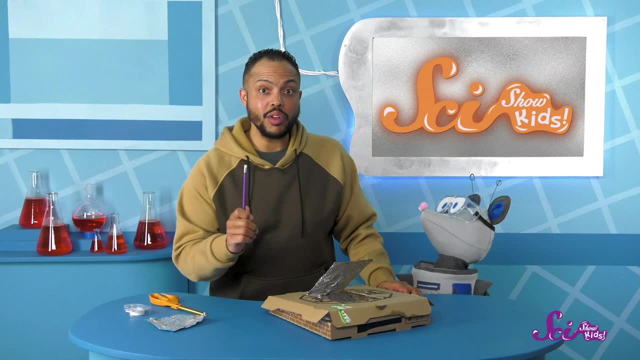 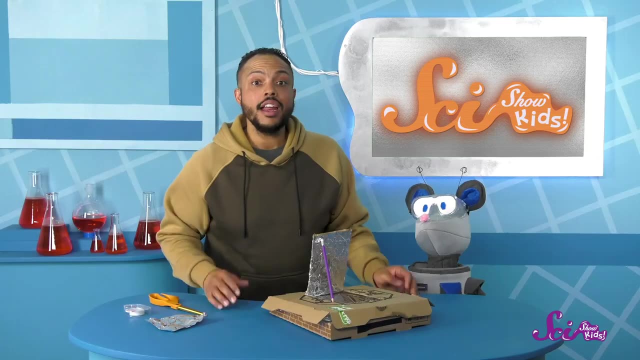 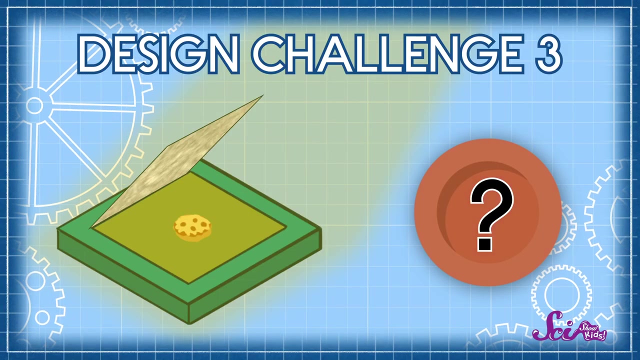 it and shoot straight into our oven. We can use this pencil to hold that lid at the right angle. Next, we'll put the food on a plate inside to cook. That leaves us with our third and final design challenge: Which color plate should we use? 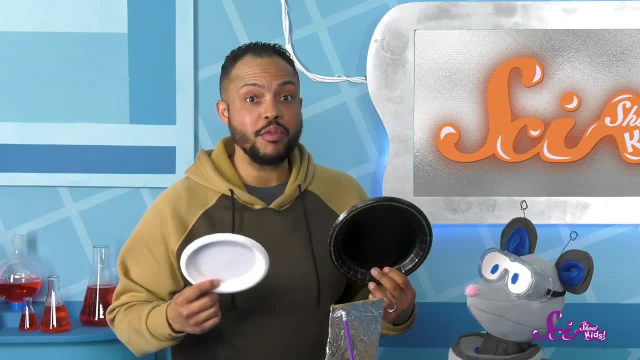 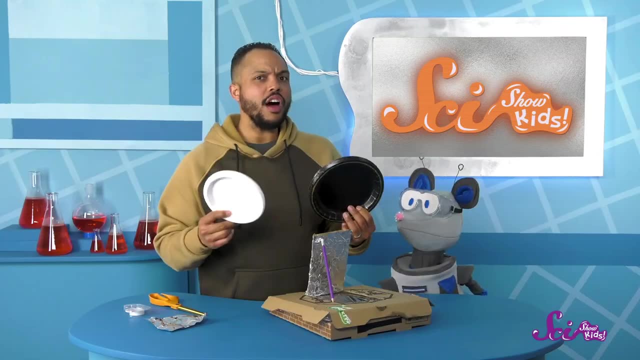 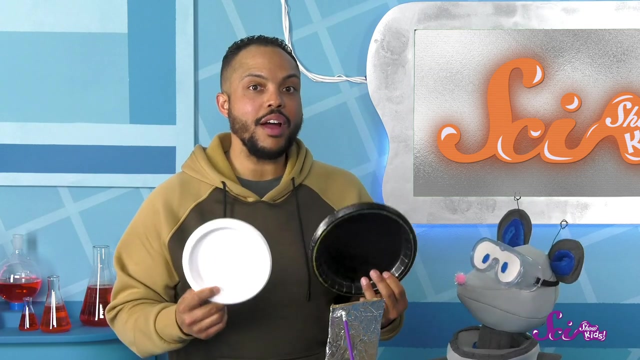 Let's see. We have a bunch of paper plates from Sam the Bat's birthday party. We have white plates and black plates. I'm glad you asked The colors matter, because dark colors heat up in the sunlight faster than lighter colors. You might have noticed this if you've ever worn a dark shirt outside in the summer. 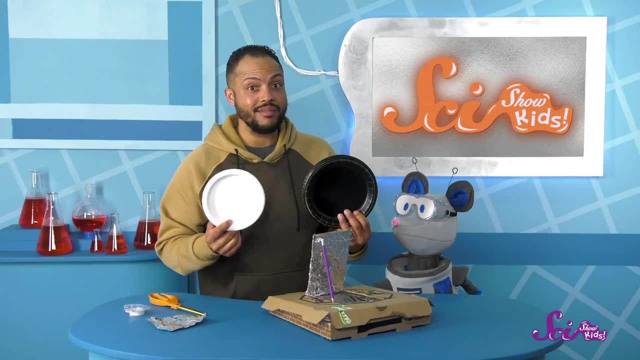 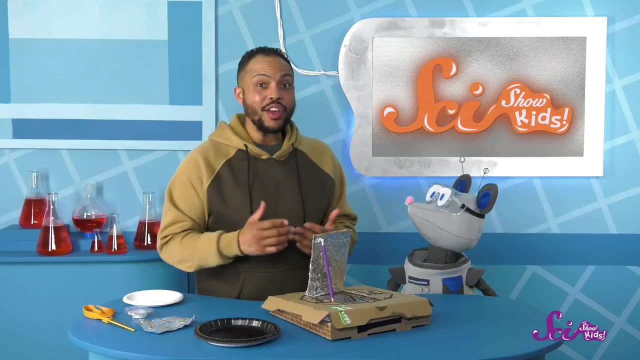 We probably want a dark-colored plate to help us heat up our food, then, don't we? I agree, Let's use the black plate. That one is darkest. It looks like we're going to need a darker plate. It looks like we're ready to test out our solar oven. 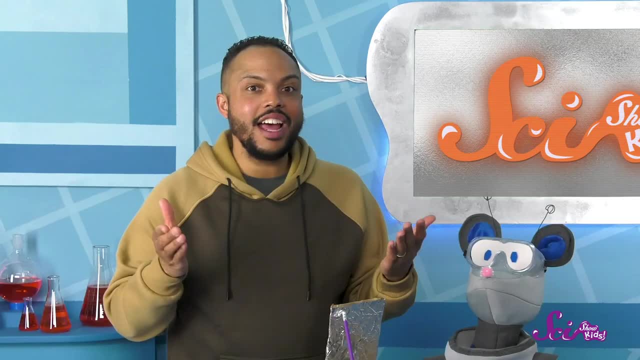 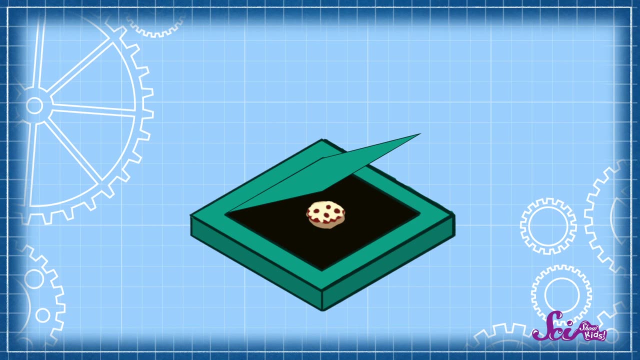 How about some pizza bagels? We're going to head outside to test our solar oven. Depending on what happens, we might make changes to our design. Maybe we'll paint the entire inside of the oven black or find a shiny mirror to help. 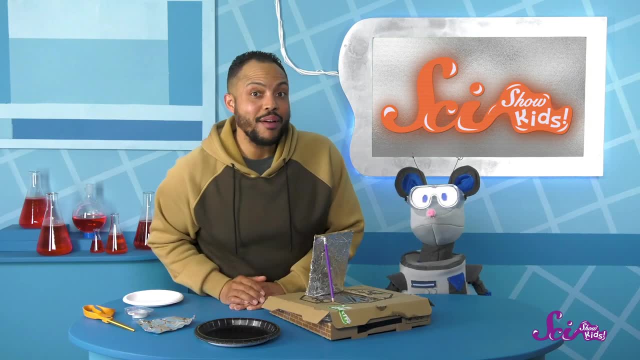 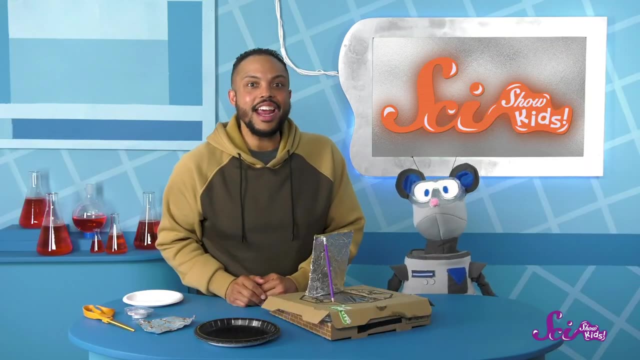 reflect more sunlight into the window. What ideas do you have to make our oven better? Ask a grown-up to help you build your own design and test it out. Good luck with your cooking And if you'd like to keep exploring with me, Squeaks, Jeff and Sam, we'll see you next time.